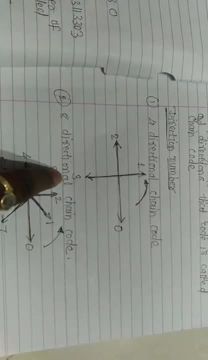 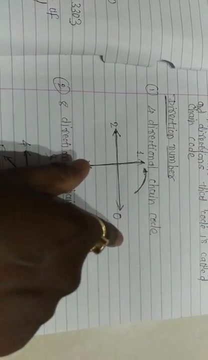 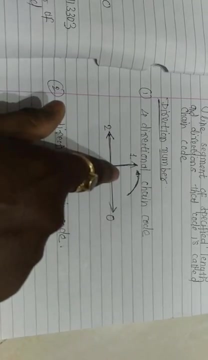 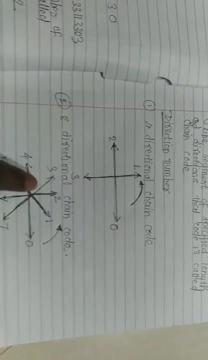 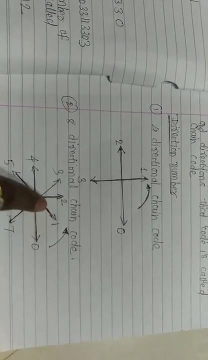 zero to seven so again we have to consider the anticlockwise direction in both four directional as well as eight directional chain code so here when we go to the right side we have to take as a zero then we go at the upside we have to take the one similarly we go at the left side we have to take it is as a two direction number and when we go at the downside then we have to take the direction number as a three similarly it the number will be considered for the eight directional chain code from the zero to seven so here we can so we can consider also the diagonal 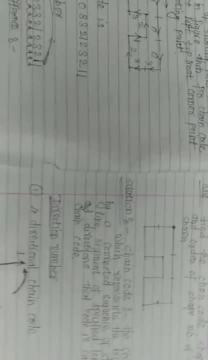 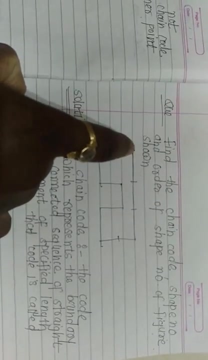 number here also then we see numerical how it is solved always the new in a numerical the starting point is given by the dark point if it is not given then always remember that this is the 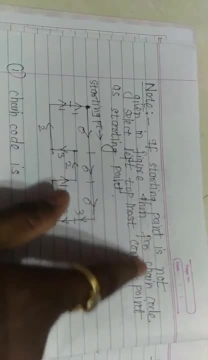 basically note if the starting point is not given in the figure then you can consider the number as a three similarly the number will be considered for the eight distance and for thewater surrounded with助 twoattAA for the former diW signal ay equals 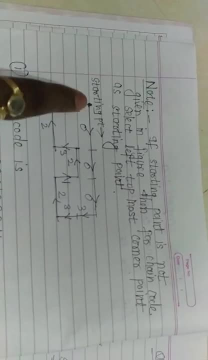 diW value for the chain code select the left topmost corner point as a starting point so this 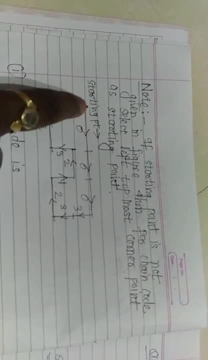 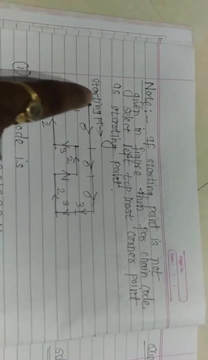 is a figure in this figure we have to take this is the left side and this is the right side so width left topmost corner will be select as the starting point this is your starting point so we have to trace the chain code from this starting point and again you have to come back at the starting point 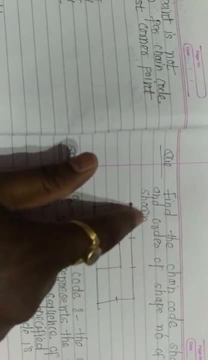 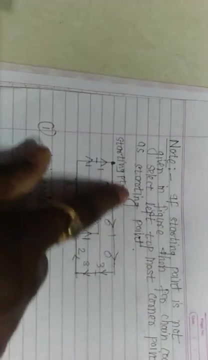 so here now in the figure there is a segment is divided toujours nombre el mismo de tres fune direction from this to this segment where to consider the second direction so in this way we have to press all the direction in the figure from the starting point so from the starting point we have to move in this direction 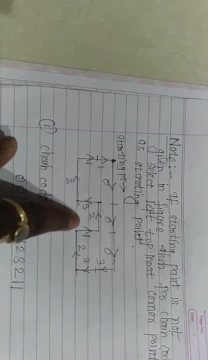 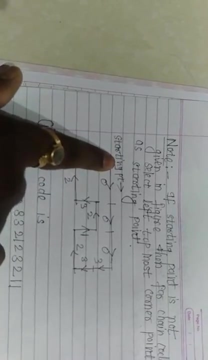 that is from in the right side then at the bottom side and then again right in this way we have to trace all the direction and again we have to come at the starting point then we have to write the chain code according to the 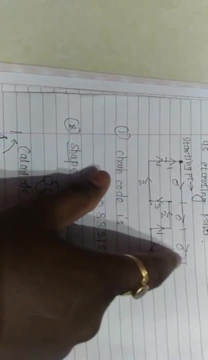 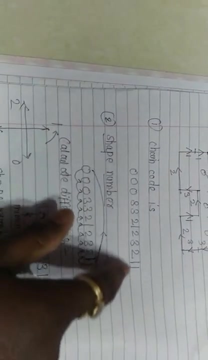 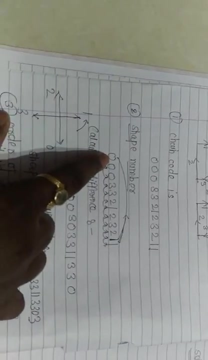 direction so this is 0 0 0 then 3 3 2 1 2 3 2 1 1 so in this way the chain code of this given figure is 0 0 0 3 3 2 1 2 3 2 1 1 then we have to calculate the shape number so for calculating